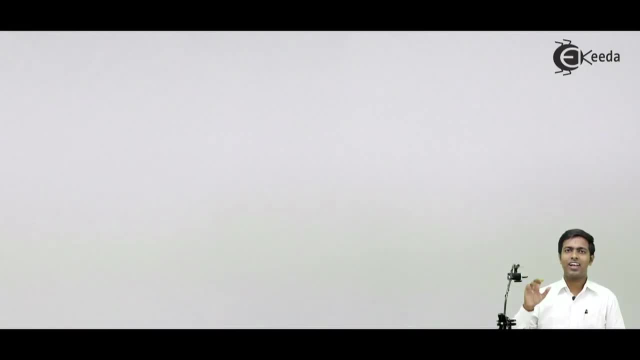 Hi, friends, now I'll ask you one question: If you want to find out square root or, let's say, cube root or the fourth root of a complex number, then how you will find. Now, as we find roots or the powers in real number, you can still find roots or powers or certain expansions of complex number. 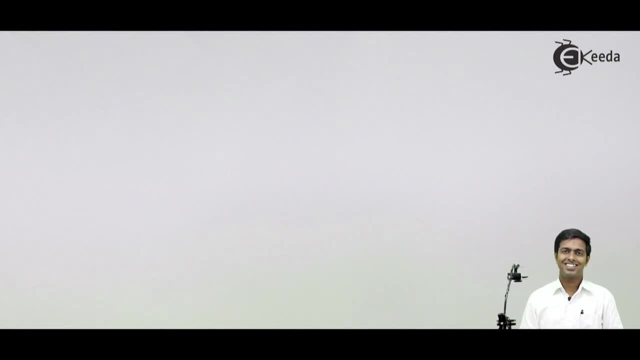 also, But how to find it? So in this topic, I'm going to teach you how to find certain expansions, roots and powers of complex number. Now, this has become possible only because of one scientist, whose name is Abraham D Moivas, So he has derived a formula. 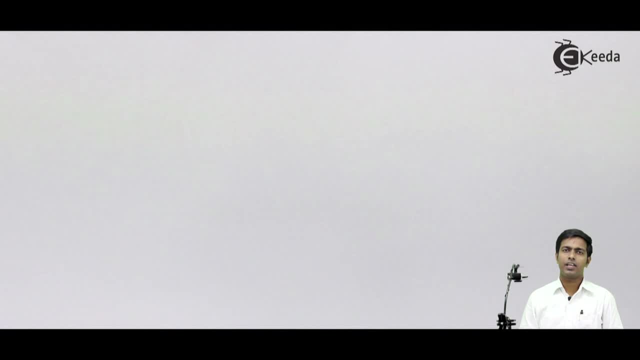 using which we can very easily find out roots or the powers or expansion of complex numbers, as we do with real numbers. So that is why this theorem is called as D Moivas theorem, So name of the topic that we are starting today is nothing but D Moivas theorem. 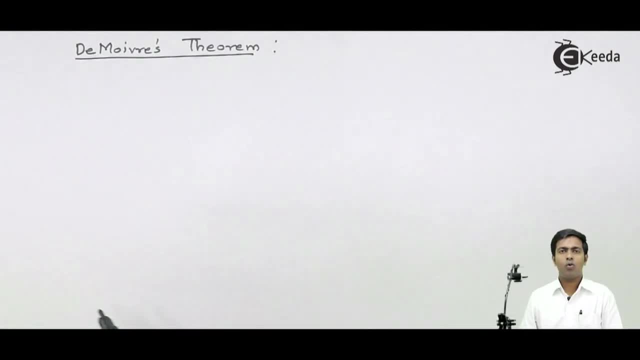 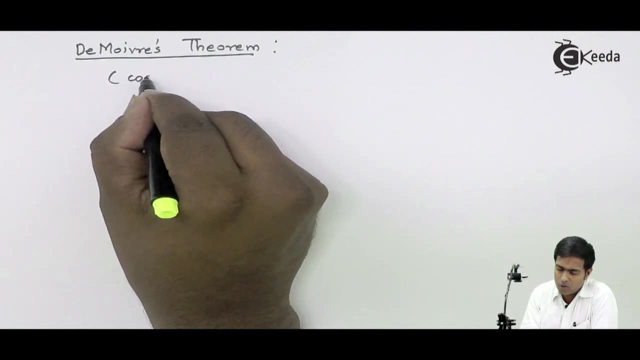 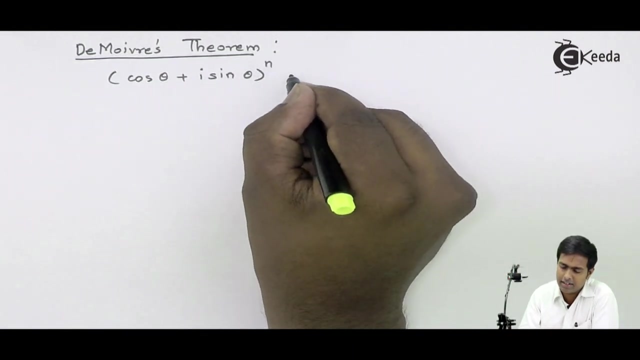 Now what Abraham D Moivas says. So according to him, if you want to find out power or root of complex number, let's say it is n, So n is any rational number. It means it can be a whole number or it can be a fraction. So cos theta plus i sine theta is a complex number. 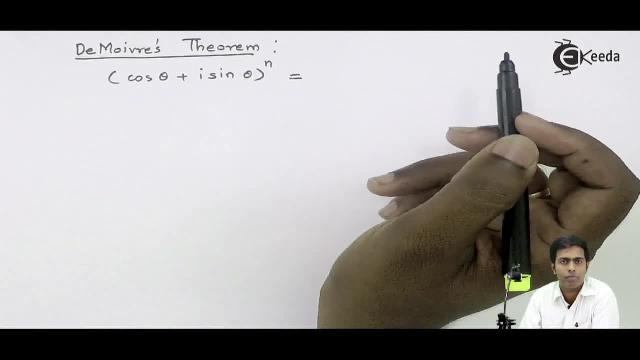 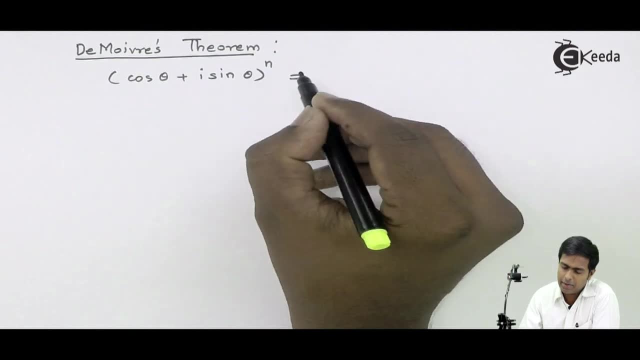 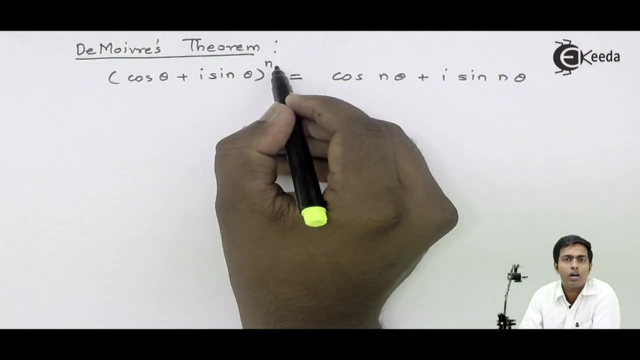 And we are trying to find out power of this complex number. So D Moivas says: whenever you are finding a power of a complex number, that time it will become cos n theta plus i sine n theta. It means your power will multiply the amplitude of complex number. Now let's take some example. 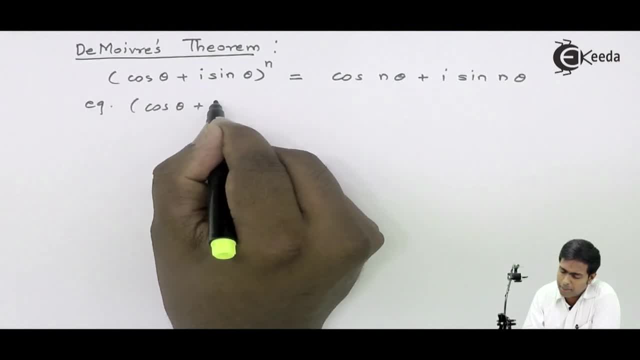 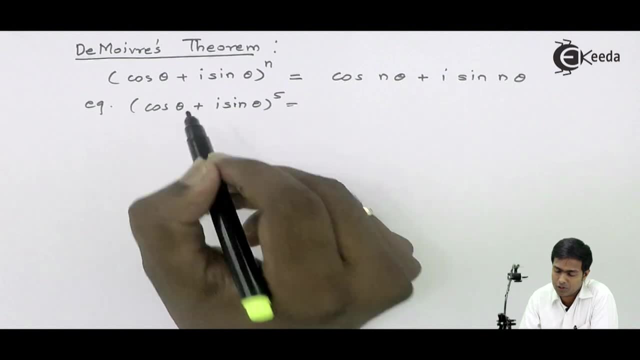 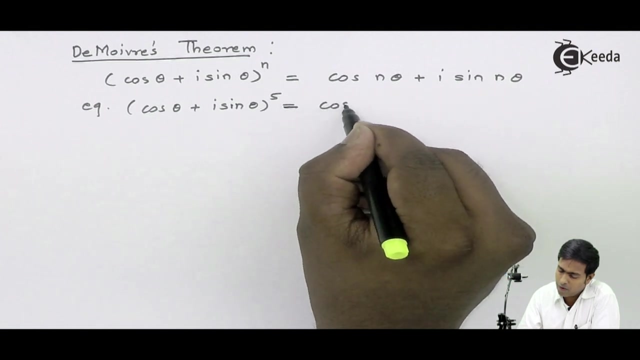 Example: if you have a complex number, let's say cos theta plus i sine theta raise to 5.. It means you want to find fifth power of this complex number. So according to D Moivas it will become cos of 5 theta plus i sine 5 theta. Suppose let's say: 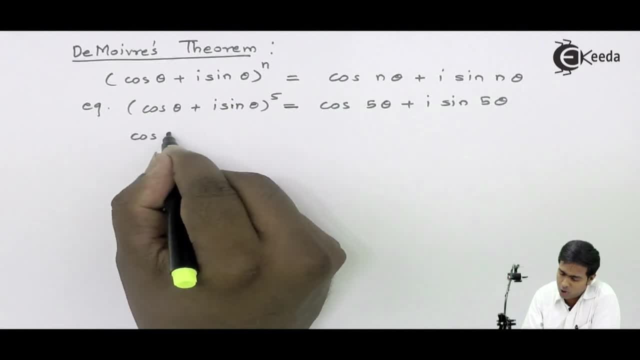 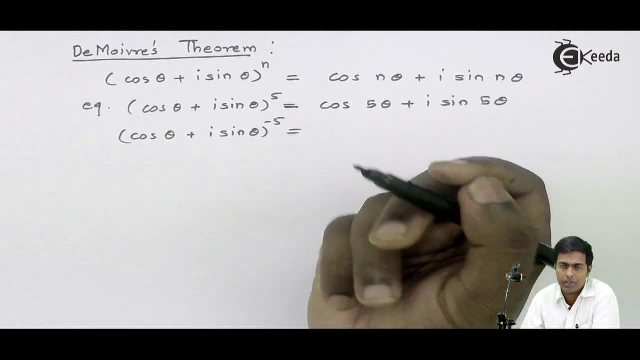 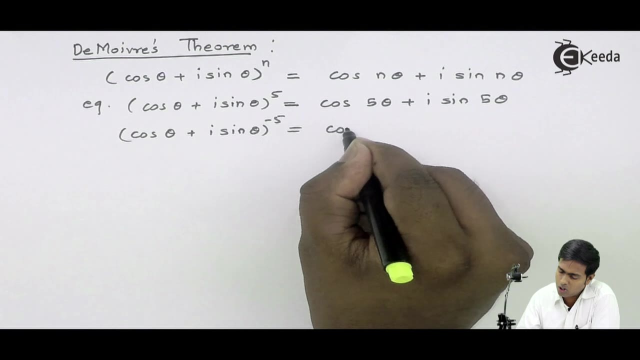 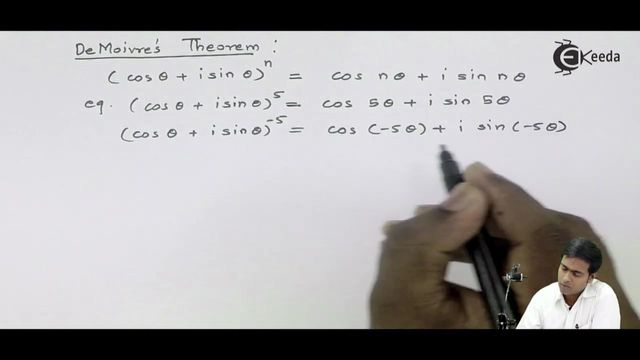 it is minus. It means if we have cos theta plus i sine theta raise to minus 5, then what will happen? Same reason: this minus 5 will multiply the amplitude of the complex number. So it will become cos of minus 5 theta plus i sine minus 5 theta. Now we all know that cos of minus theta is cos. 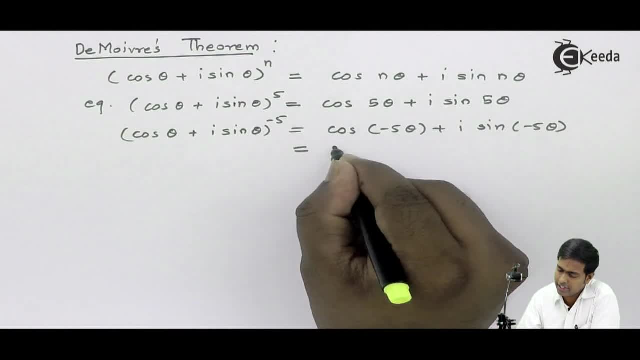 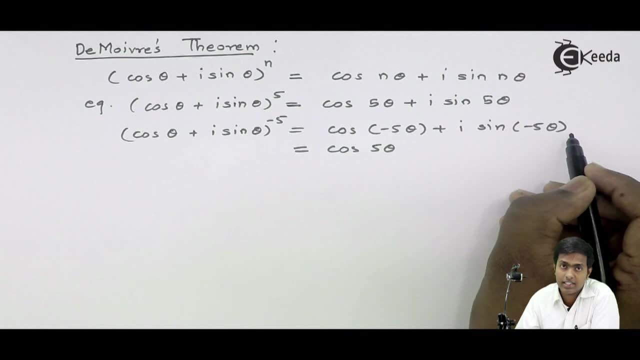 theta. Hence cos of minus 5 theta is: yes, it is cos 5 theta. Similarly, sine of minus 5 theta is minus sine 5 theta, So it will become minus i sine 5 theta. So it means, if you want to find out, negative power of. 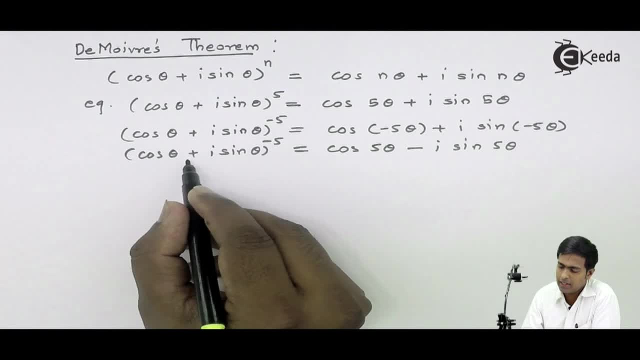 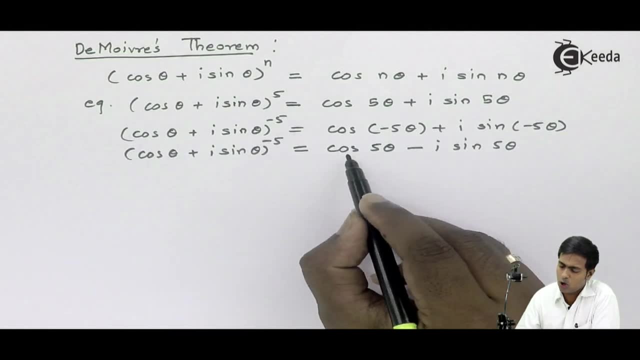 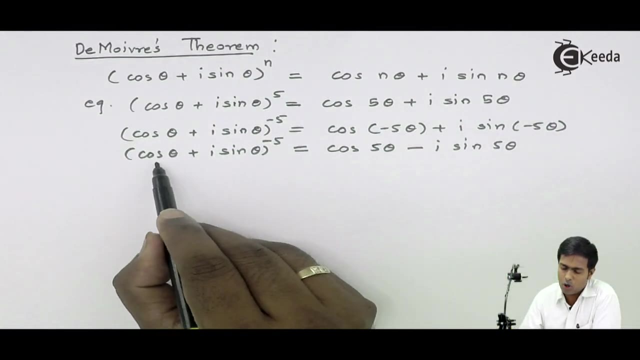 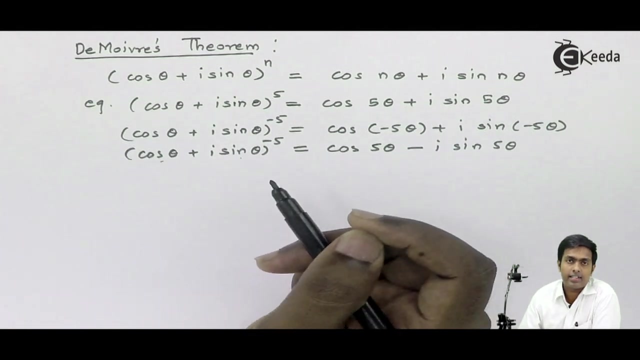 any positive complex number, then the sine will become negative, and vice versa is also true. It means cos phi theta minus i sine phi theta is given to you, then you can write it down as cos theta plus i sine theta whole raise to minus 5.. Now let us say, let us take some fraction. So 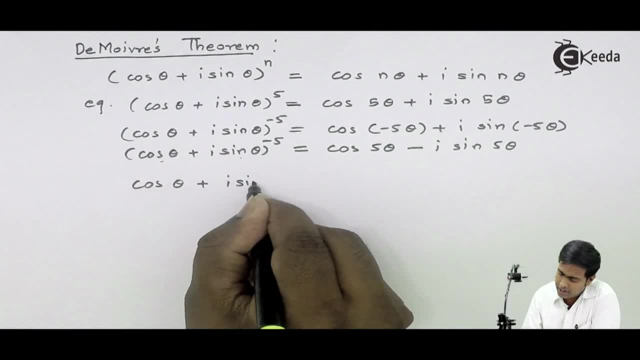 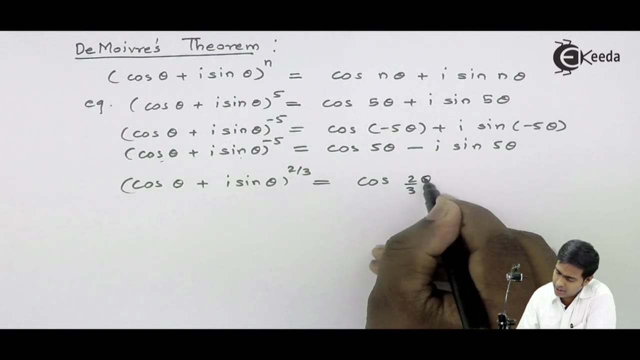 if it is cos theta plus i sine, theta raise to 2 by 3.. In this case what will happen? Same rule: 2 by 3, it will multiply this theta, So it will become cos of 2 by 3 theta plus i sine. 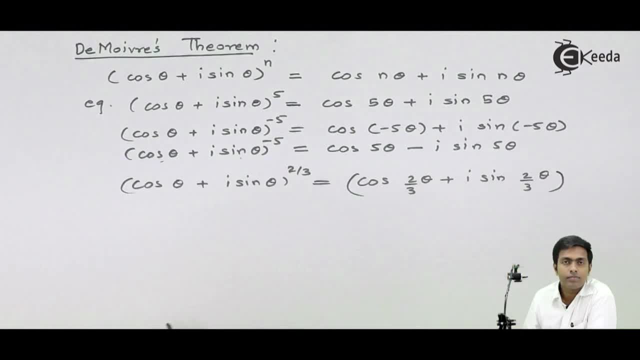 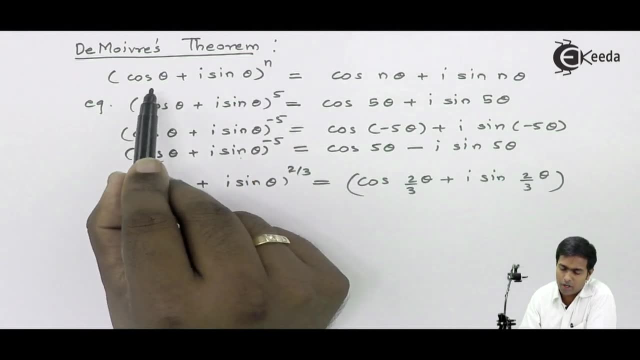 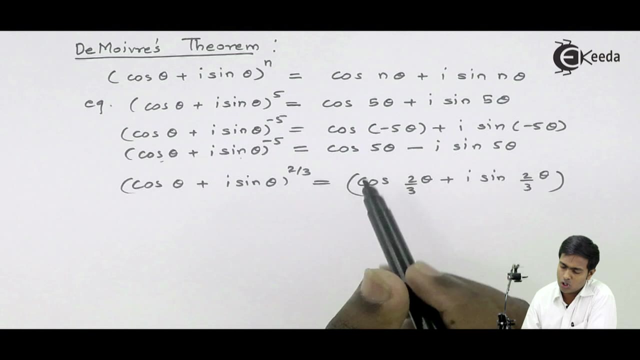 2. So, according to De Moivre's, whatever is the power or the root that you are finding for any complex number, that power or root will multiply amplitude of the complex number. So, using this theorem, we will see some numericals. and let us solve some numericals using the result of De Moivre's.